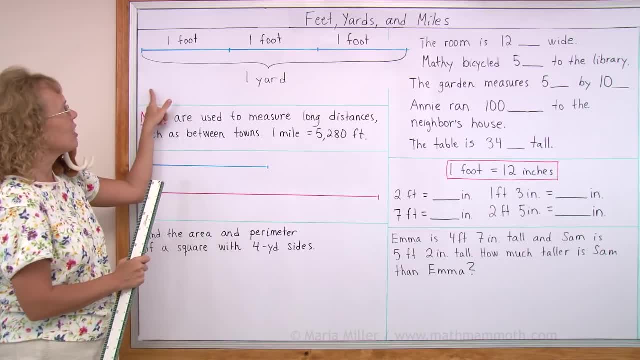 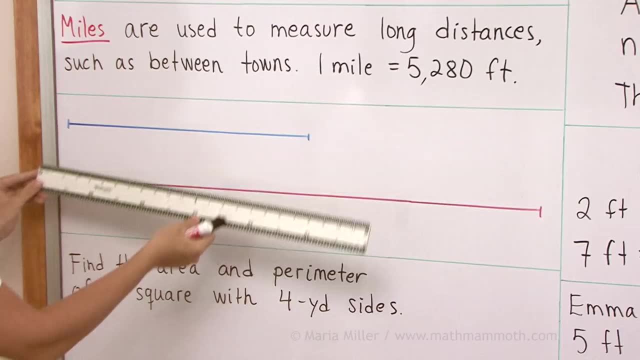 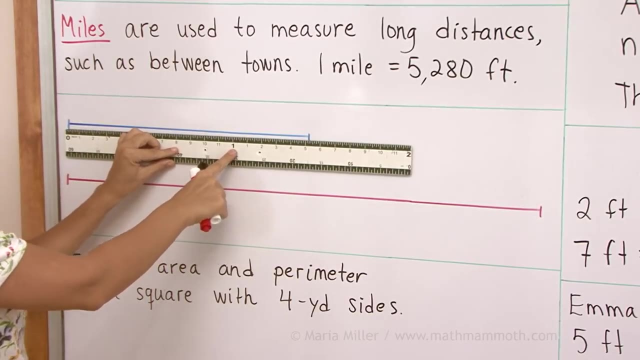 long units And the smallest ones were inches, then was foot, then yard, okay- And then lastly miles. Here I have 2 lines that I'm going to measure And, as you can see, this one is more than 1 foot long, because 1 foot is here. 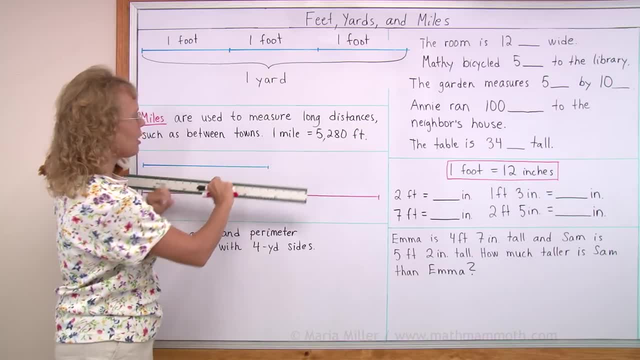 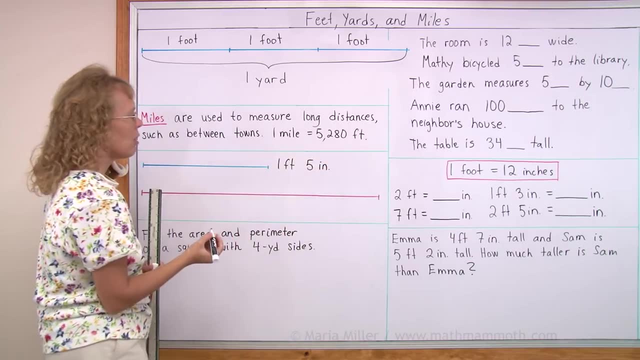 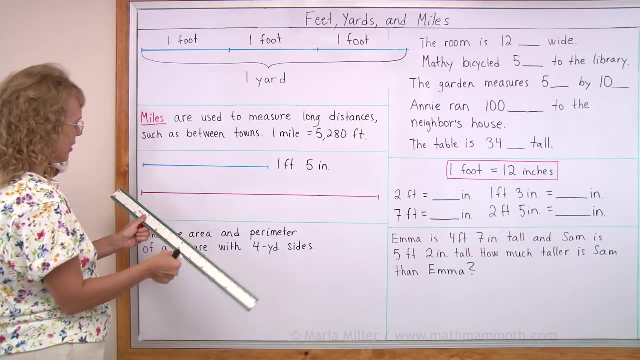 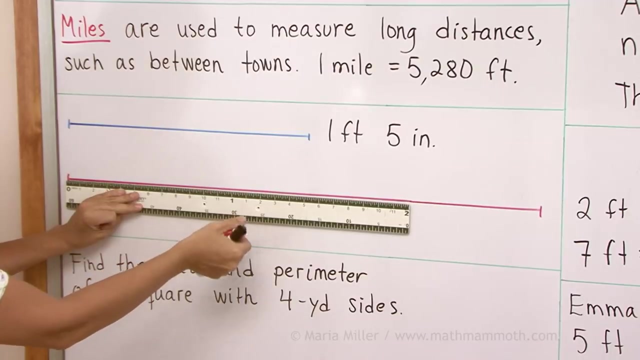 So after 1 foot, I have 5 inches. So it is exactly 1 foot 5 inches, And this is how I can abbreviate: foot as ft and then inch as in, as you know. And then this second line is longer than my ruler. So what I will do is I will mark here at 2 feet, then take my 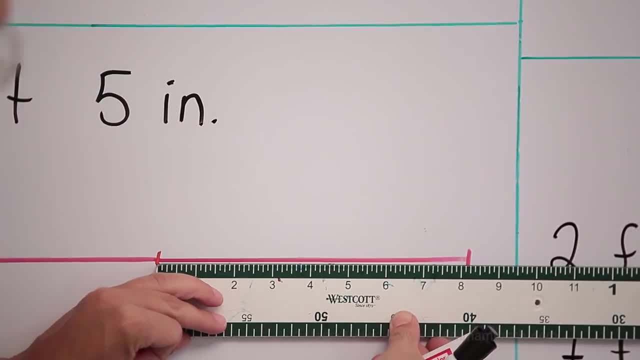 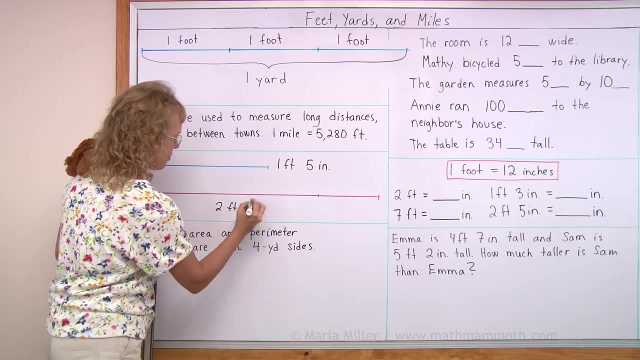 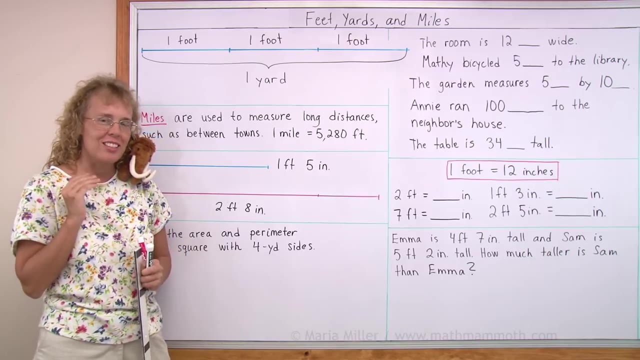 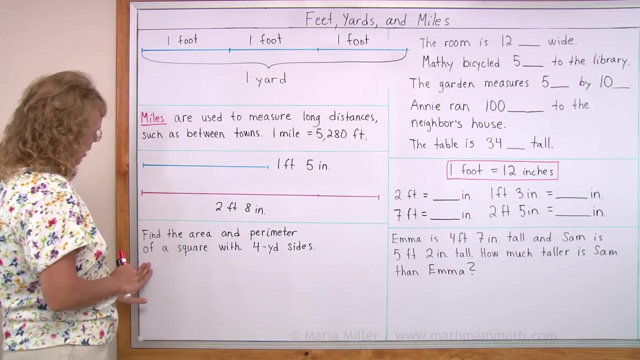 ruler and it is 8 inches, Or in other words, 2 feet 8 inches. And you also, I want you to measure, practice measuring things: how high they are, how tall or how wide or how long different things are in feet and inches. Over here we're going to find the area and 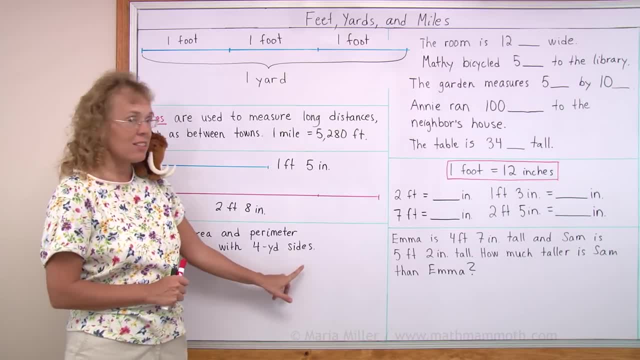 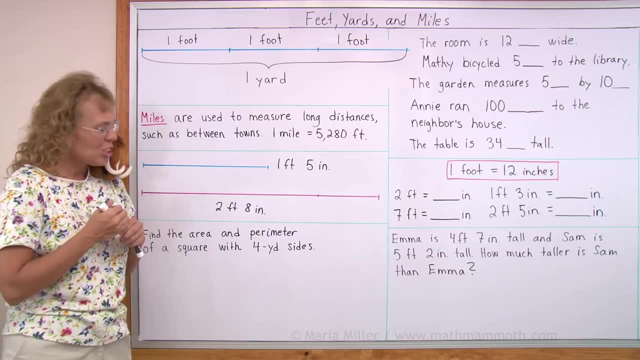 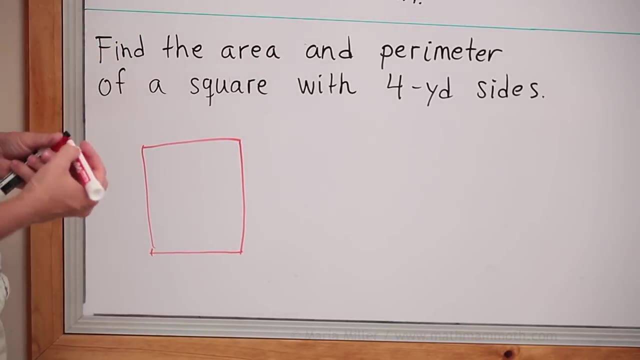 perimeter of a square, Yard sides. okay, It's a geometry problem talking about area and perimeter and a square. So draw a sketch, just a little picture, kind of help. you think Some kind of a square, a little floppy, But it doesn't matter, it helps. you think okay, And then you can mark. 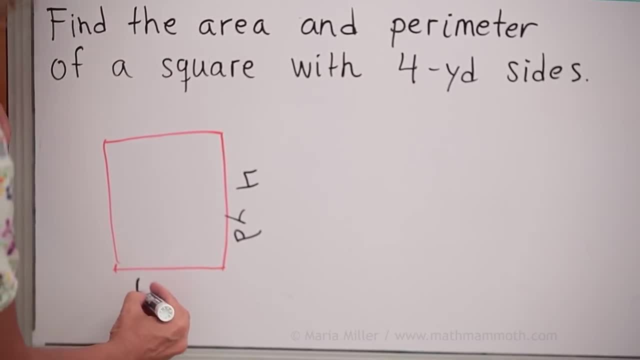 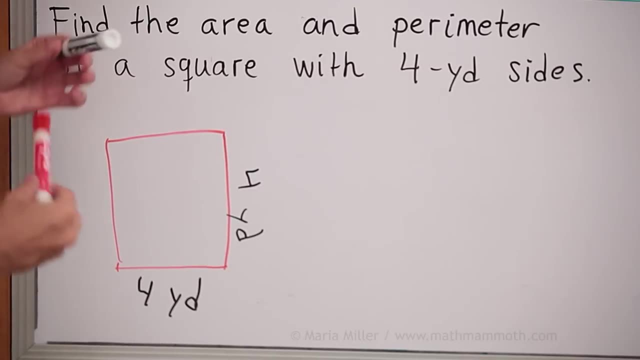 on it what you know: 4 yards, and this side is 4 yards. So what is its area? For the area, you remember? I could mark this mark off these sides with the 4-yard increments, I could draw these lines and get the grid And I could count the squares inside, Or I can 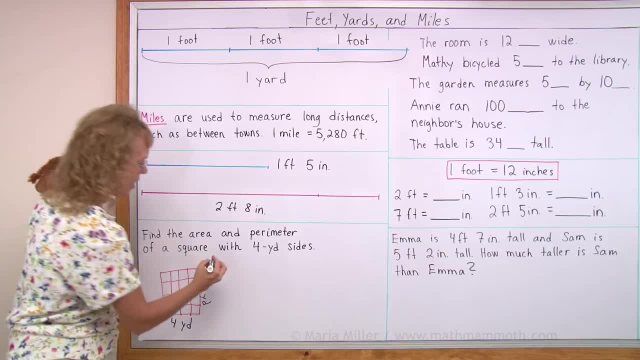 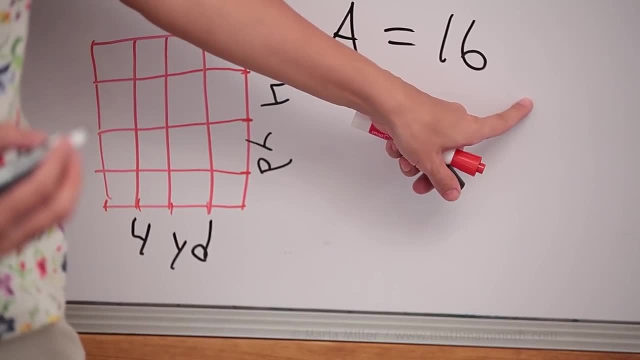 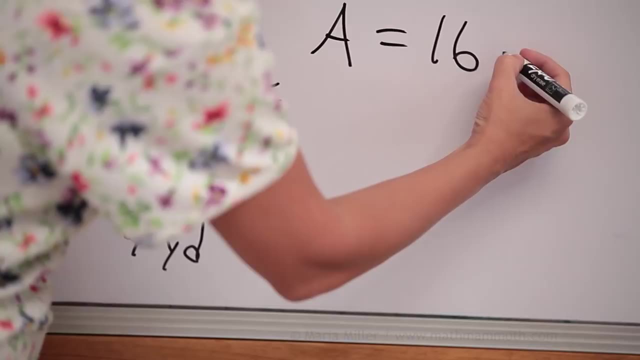 multiply, which is quicker, 4 times 4.. The area A for area, the area is 4 times 4, gives us 16.. What unit will I put here? Area is always measured in square units, So I have to put here square yards or yard. 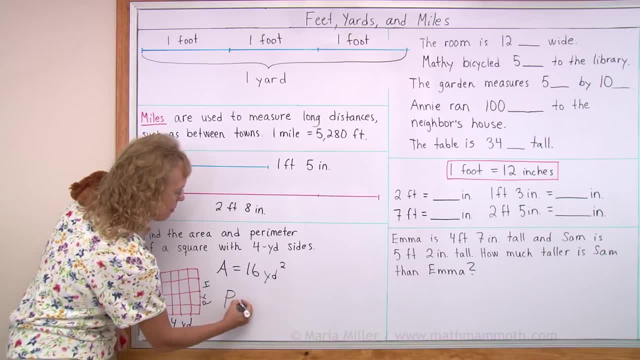 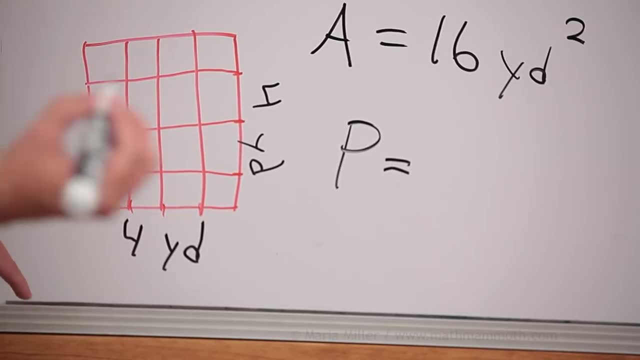 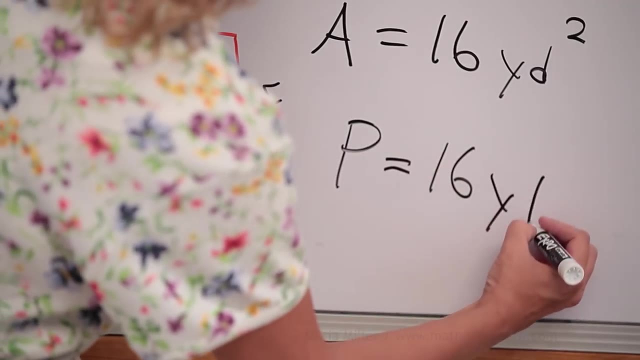 and then this little 2.. And then the perimeter. you go around the figure 4 and 4, and 4 and 4.. That's 4 times 4, 16 too. But this time what unit will we put here? The same as here. 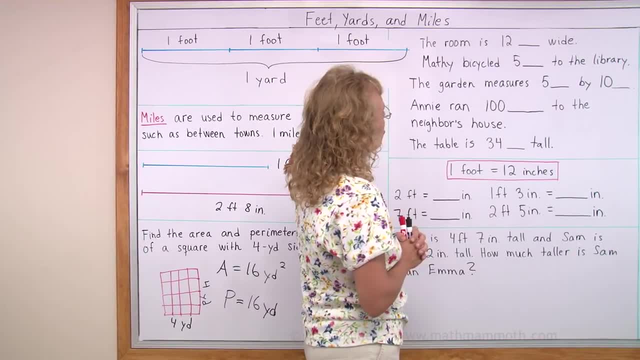 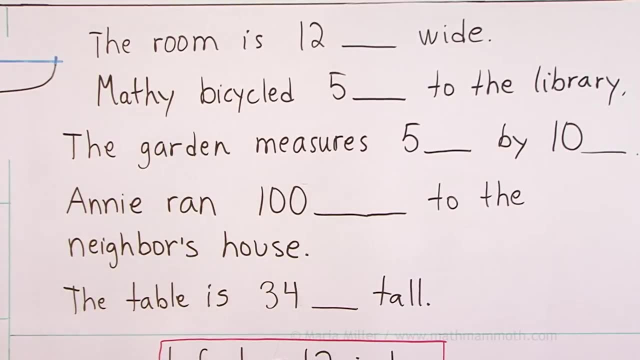 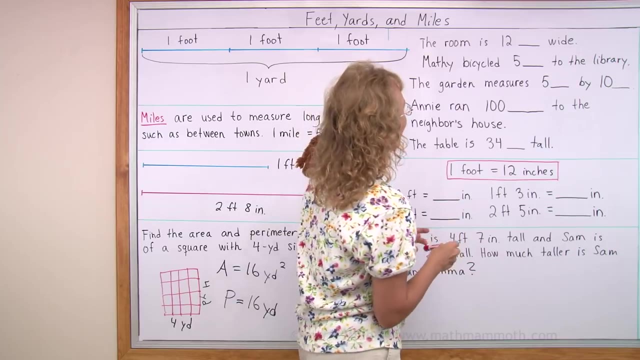 yards. Alright, Over here, our task is to fill in the blanks so that it makes sense. okay, The room is 12 watt wide. A unit Miles Centimeters Feet. What 12 inches won't work. that would be pretty. 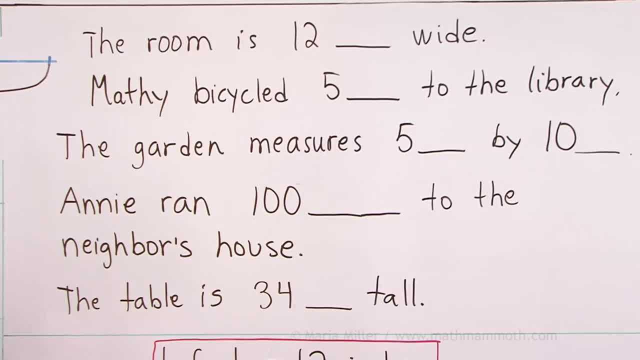 little room. unless it was a dollhouse, Then 12 inches might work. If it is a normal room, I think we need to use feet. Matthew bicycled 5 something to the library. Okay, 5 inches, 5 feet. 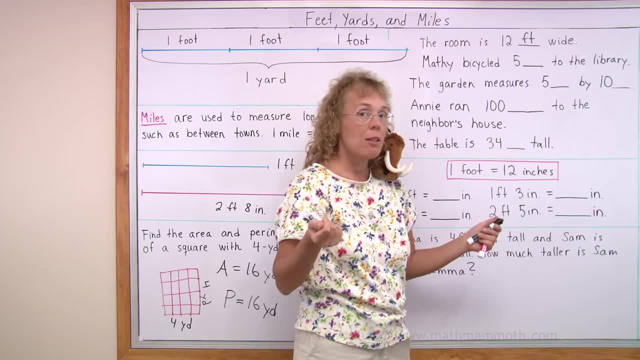 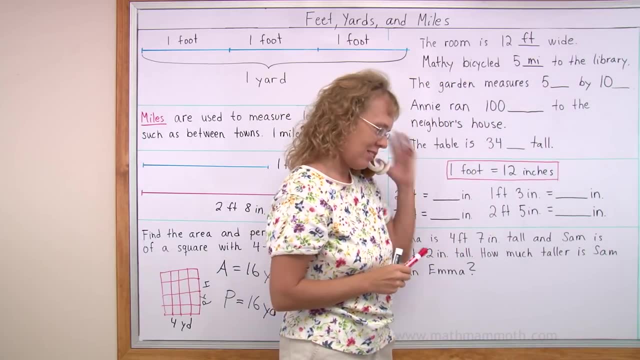 5 yards, 5 miles, 4 km for miles, вроде, Aha, miles, of course. Matthew, what kind of books did you get? 5 congestible? Oh, okay, I should have biggest, Yeah puzzle books. 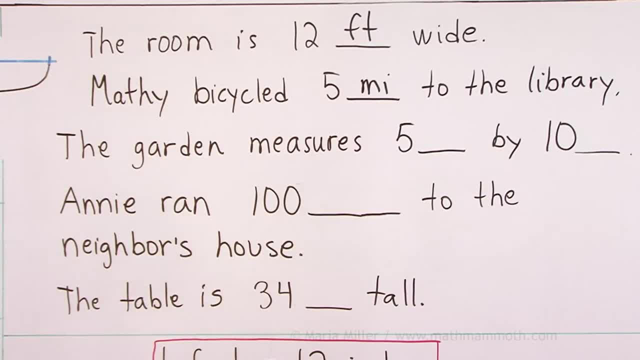 The garden measures 5 something by 10 something. So 5 inches- no, can't be inches, can't be miles, But it could be feet or yards. However, even 5 feets or yards could be 5 feet, even. helped a bit, because if 51 inches is there, there is no Maximum Wing: 17 inch, number 5?, 85 inches, schlea, 60?, 65?, 75?, 66?, 60?, 75?, 16?. 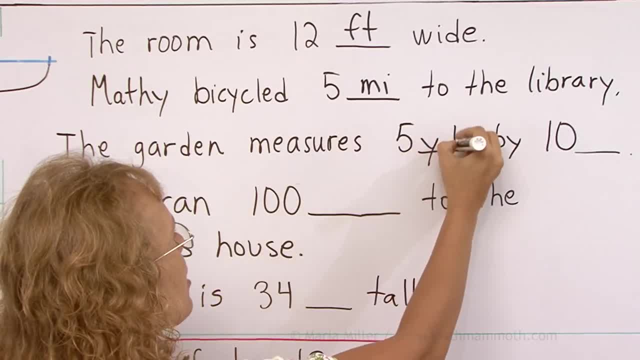 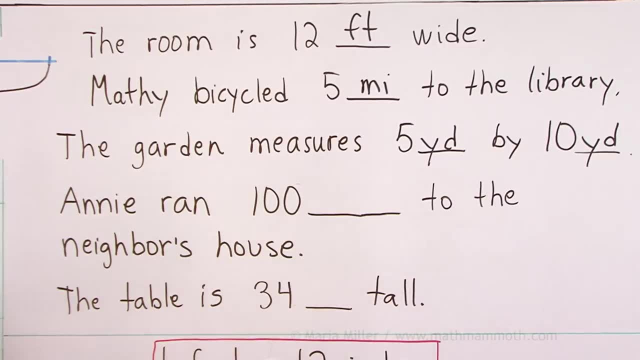 90%. 27? feet is not a very big garden, so I think it might be yards. Let's put yards here. that works best. Annie ran hundred something to the neighbor's house Here. two units are possible. It could be she ran 100 feet, but then again maybe she ran. 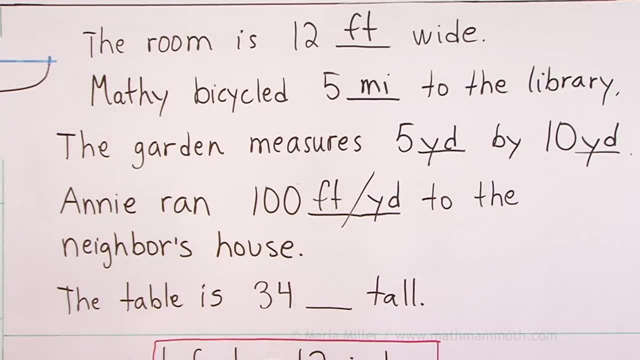 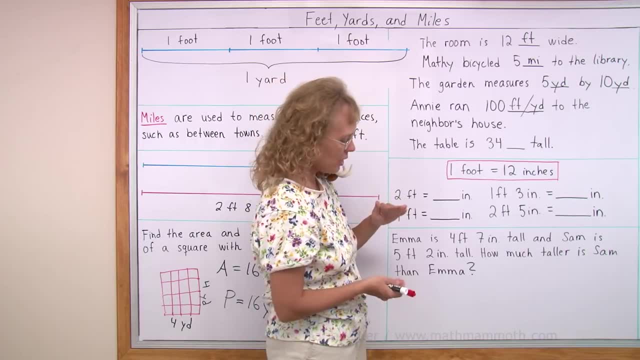 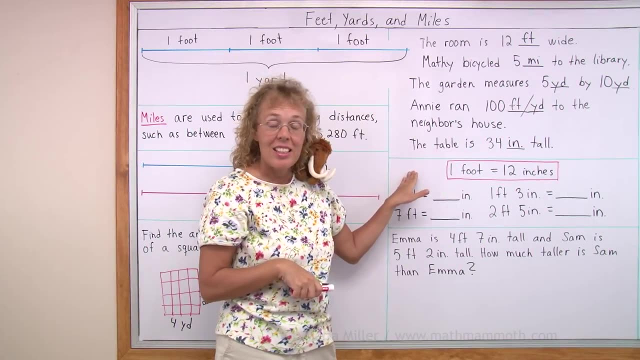 100 yards, three times as much. The table is 34 something tall. This could even be centimeters, but it would be a pretty, a pretty small table. I think inches work best here, Don't you think? Lastly, we're gonna do some conversion problems. 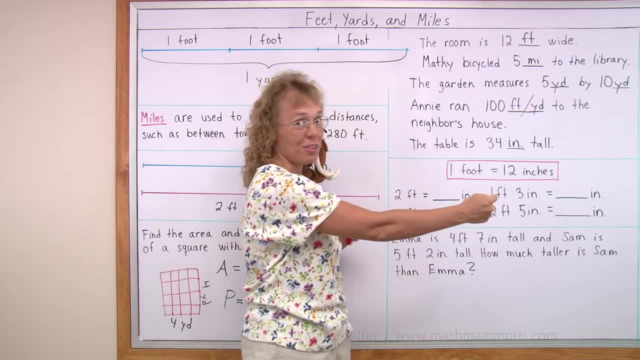 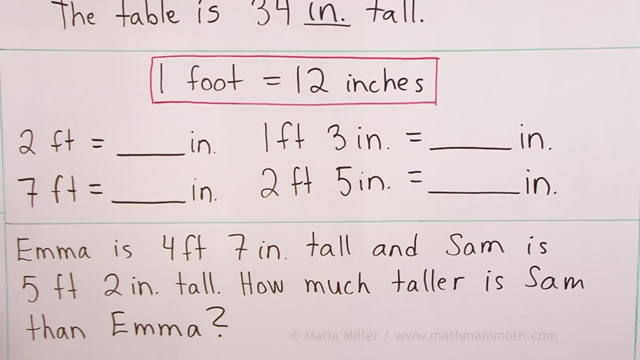 One foot is 12 inches, like I told you, and you saw it on the ruler right. So how about two feet? How many inches would it be? If one foot is 12 inches, two feet is 24 inches. yes,